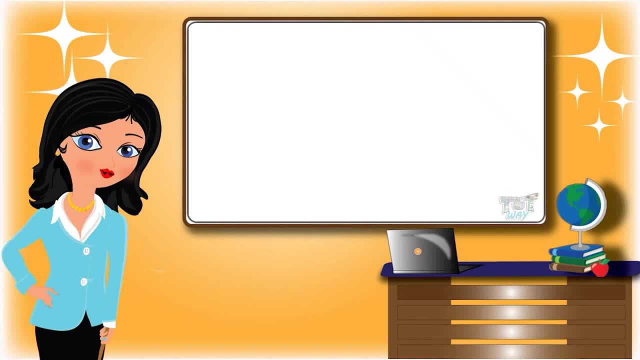 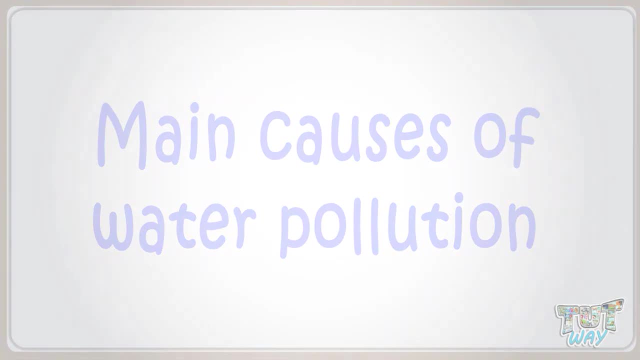 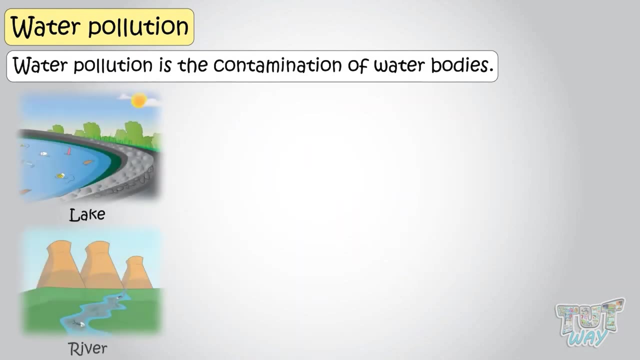 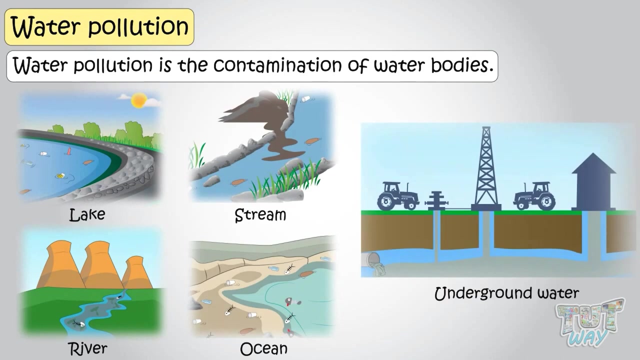 Hi kids. Today we will learn the main causes of water pollution. So let's get started, Kids. water pollution is a contamination of water bodies like lakes, rivers, streams, oceans and even the underground water, And this pollution makes the water in water bodies unsafe for use. 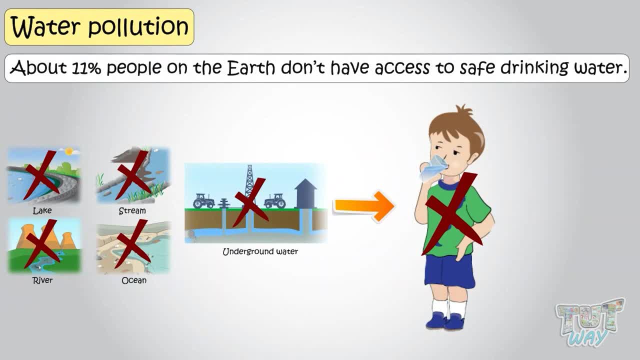 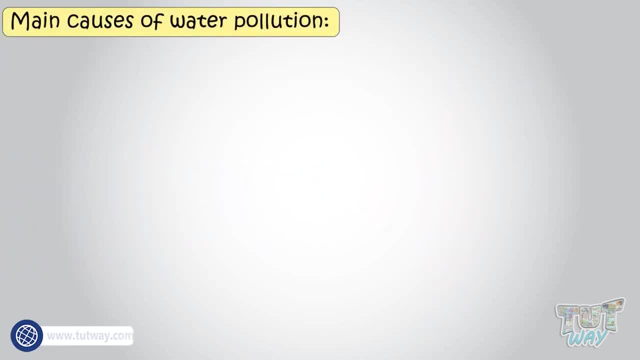 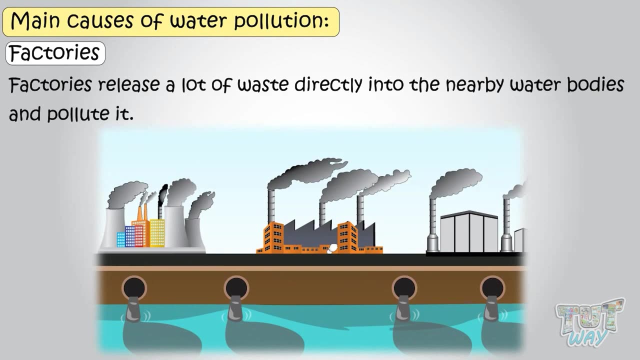 About 11% of people of the earth don't have access to safe drinking water. Now we will learn what are the main causes of water pollution. Most factories, industries, manufacturing units release a lot of waste directly into the nearby water bodies and pollutes it. 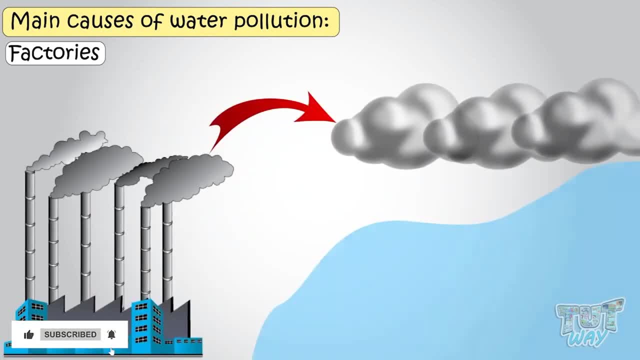 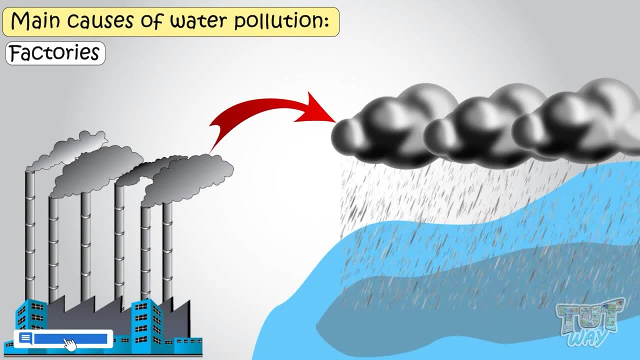 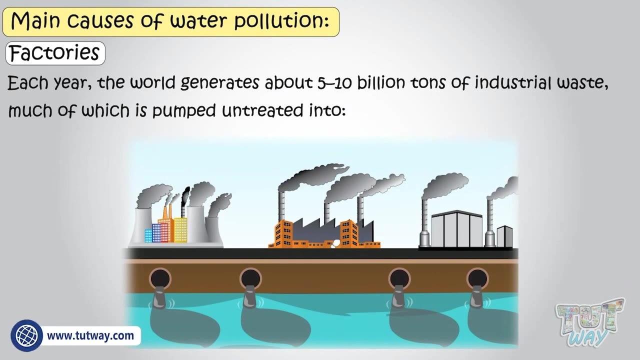 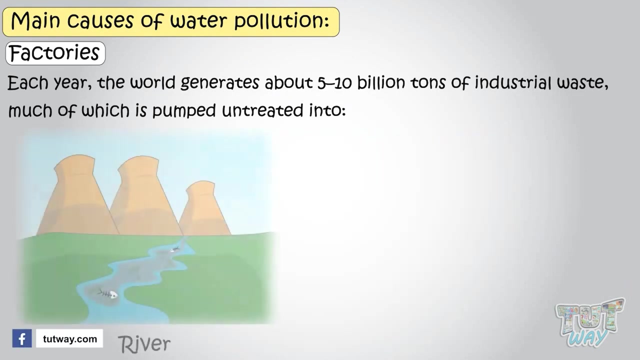 Even the smoke released by chimneys of factories, too, Reaches the water- The water along with polluted rain, And so pollutes water. Each year, the world generates about perhaps 5 to 10 billion tons of industrial waste, And much of which is pumped untreated into rivers, oceans and other waterways. 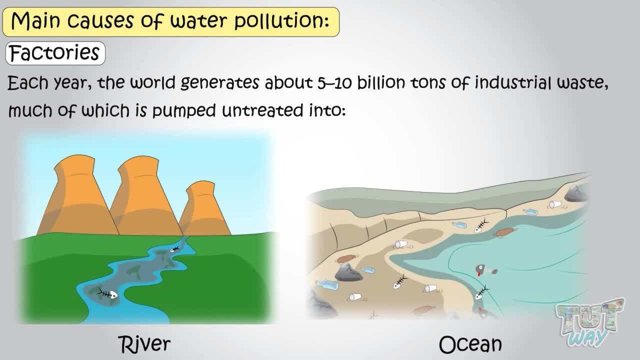 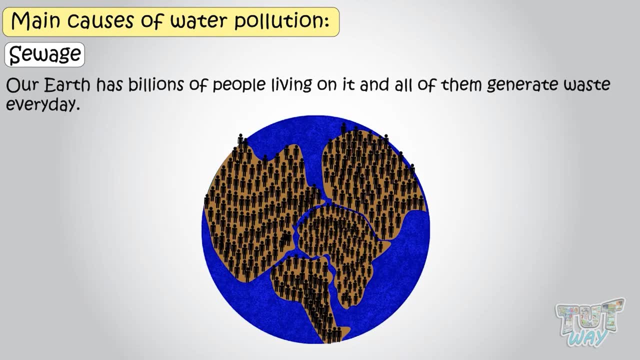 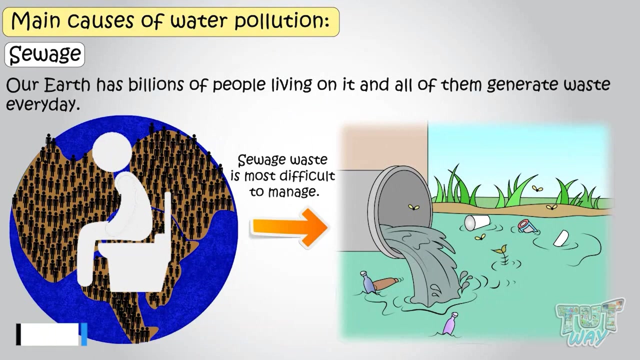 And it is the main reason behind the water pollution. Next is the sewage. Our earth has billions of people living on it And all are generating waste every day, And managing this waste is a very big problem for all of us. And out of that, sewage waste is most difficult to manage. 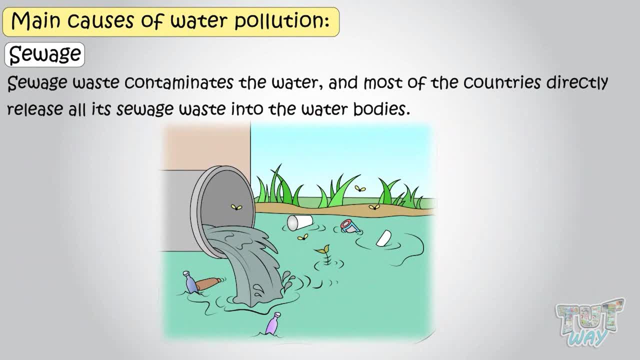 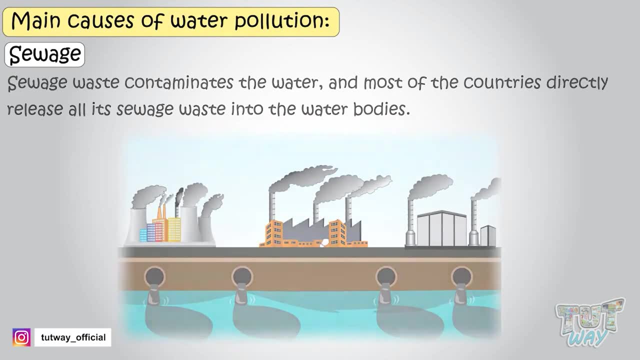 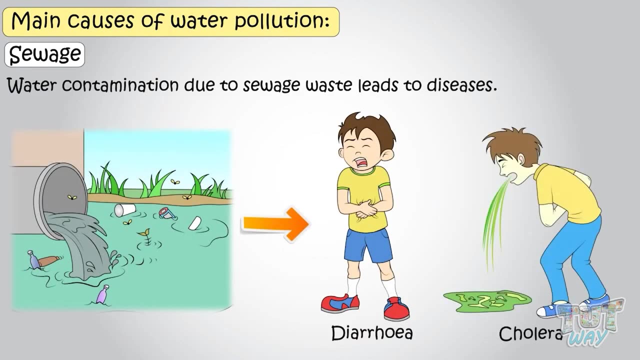 Sewage waste contaminates the water And most of the country's directly releases all its sewage waste into the water bodies. And water contamination due to sewage waste leads to diseases like diarrhea and cholera, And according to WHO, that is, World Health Organization, water-related diseases can kill 135 million people by 2020.. 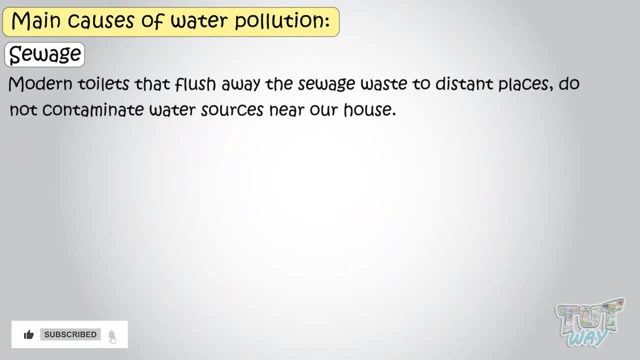 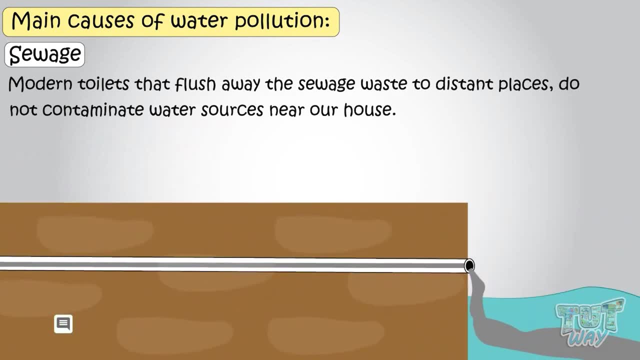 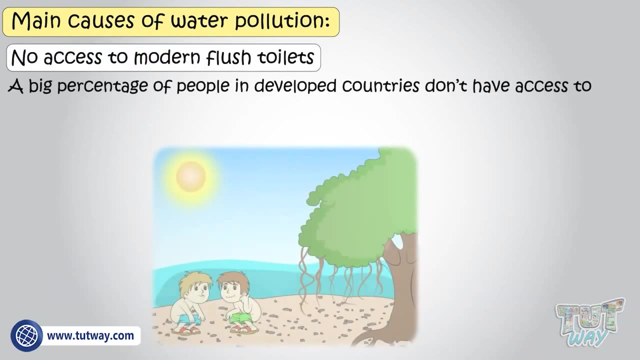 In case of developed countries, we have modern toilets that flush away the sewage waste to distant places And does not contaminate water sources near our house or our environment. But in case of undeveloped countries, a big percentage of people don't have access to modern flush toilets. 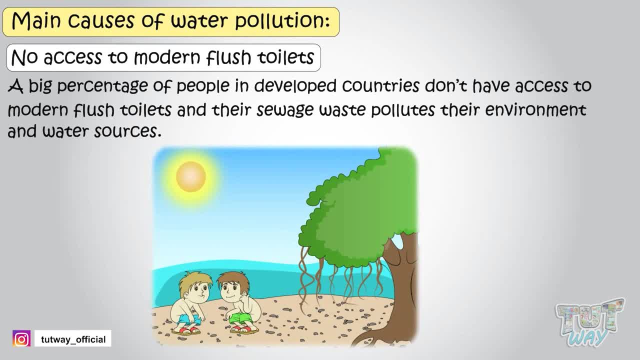 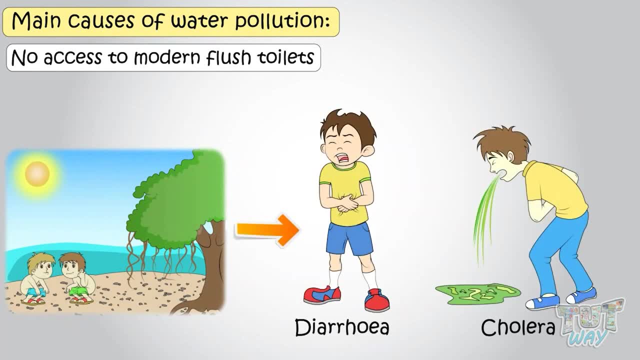 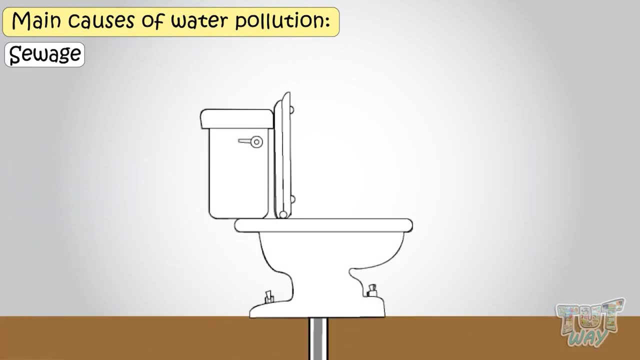 And their sewage waste pollutes their environment and water sources, Which leads to diseases like diarrhea and cholera. But that's not all. Even in the case of modern countries, where there are modern flush toilets, sewage is disposed at some distant place. 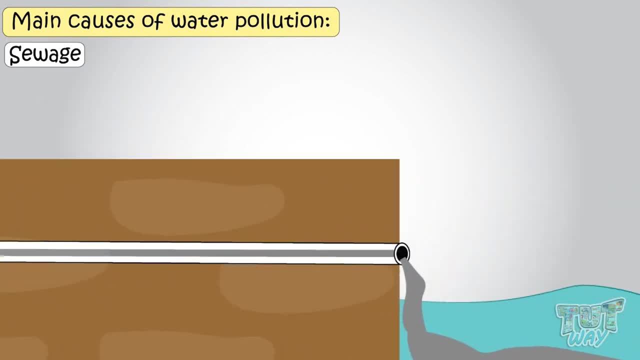 Like it can be pumped into the sea or river, So it's too polluting the big water bodies. Sewage waste is pumped into the sea through big pipes untreated, Which contaminates the oceans and seas Around. half of all ocean pollution is caused by sewage waste. 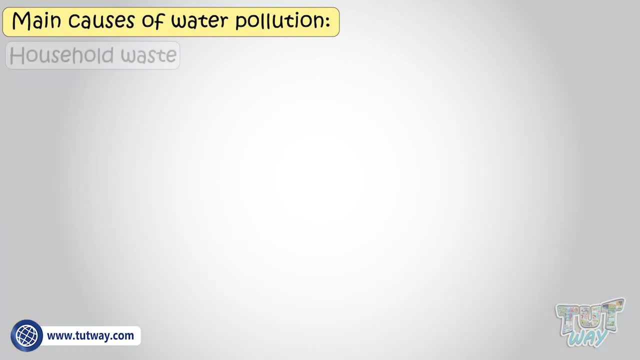 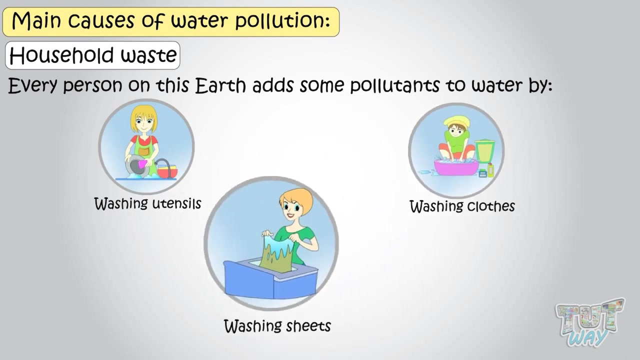 And the waste water. Next, it is household waste. Every person on this earth adds some pollutants to water, As utensils, clothes and sheets are washed in every house using some kind of detergent and soap. People bathe using soaps and shampoos. 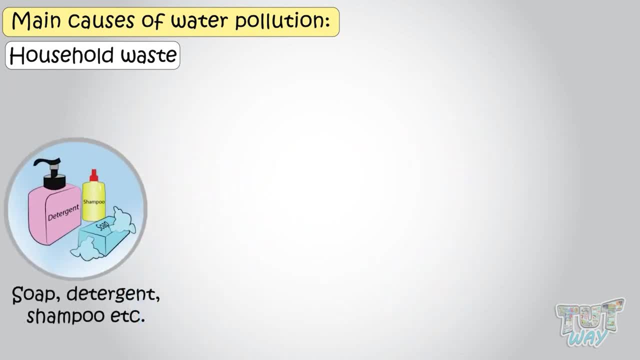 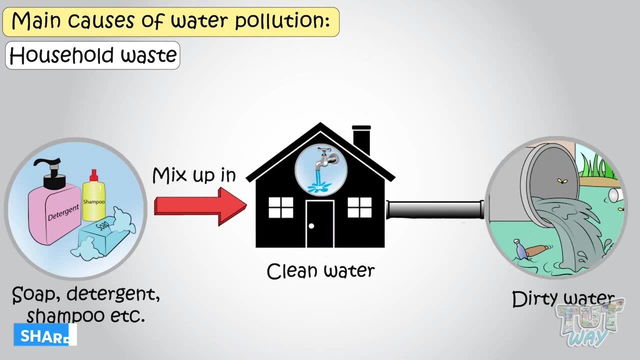 All these soaps, detergents and shampoos mix up in clean water And changes the clean water into dirty water That ultimately reaches some water bodies Through long pipes and contaminates the water. Highway runoffs- Highways are made up with a lot of toxic chemicals. 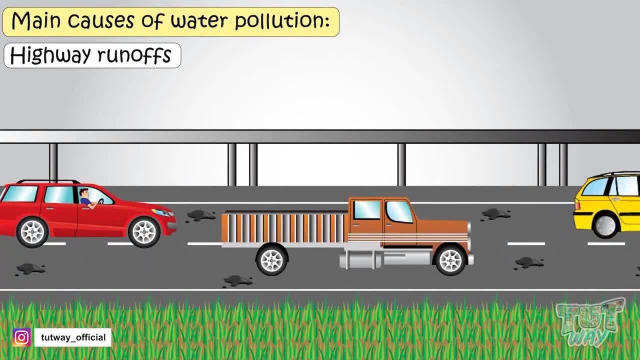 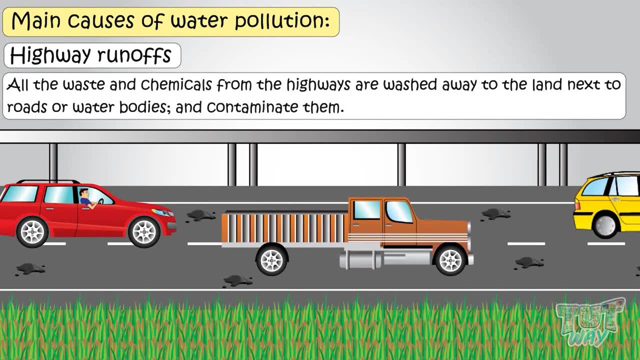 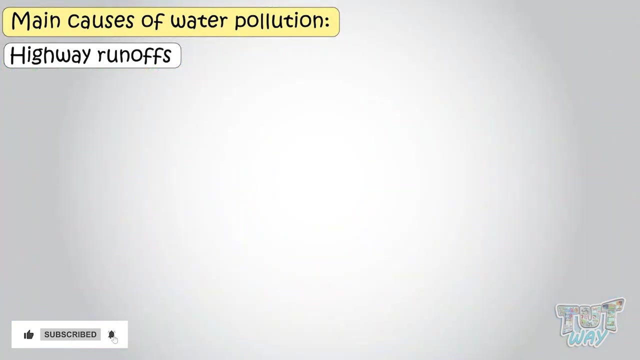 And there is spilled fuel, brake fuels and other wastes and dust From the tires. All the wastes and chemicals From the highway are washed away To the land next to roads or water bodies And contaminate them. It has been estimated that in one year 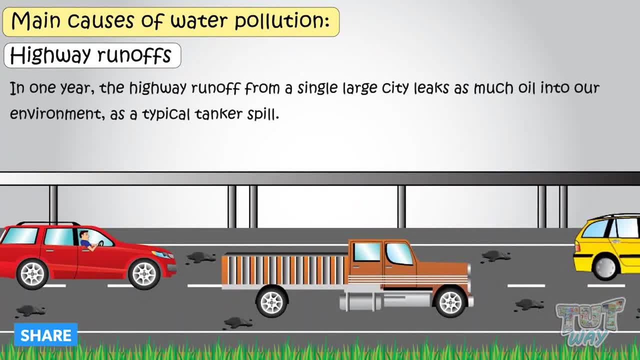 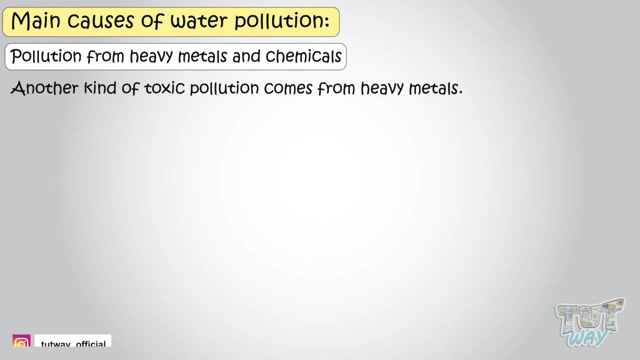 The highway runoff from a single large city Leaks as much oil into our environment As a typical tanker spill. Pollution from heavy metals and chemicals. Another kind of toxic pollution comes from heavy metals Such as lead, cadmium and mercury. Lead was once commonly used in gasoline. 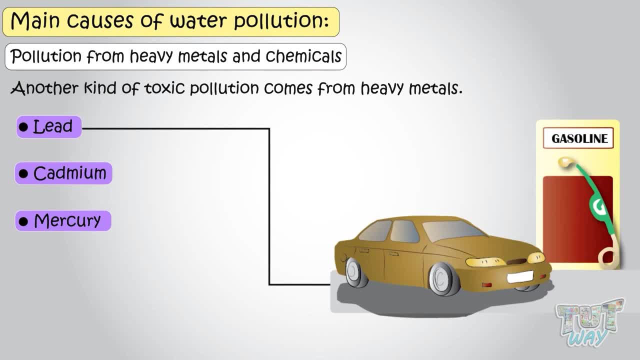 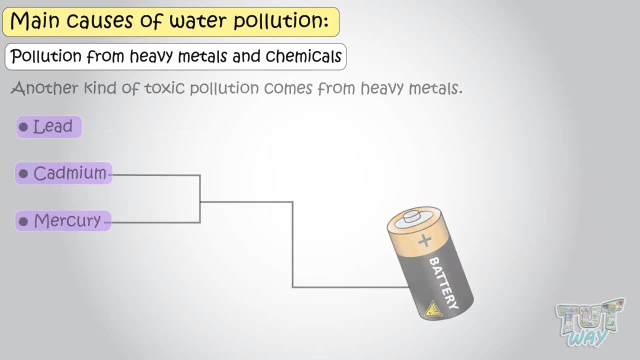 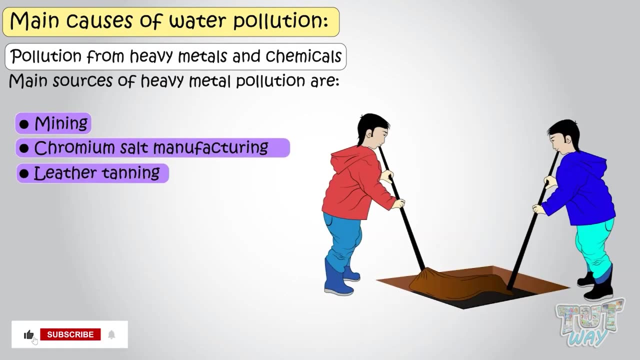 Though its use is now restricted in some countries, Mercury and cadmium are still used in batteries. Main sources of heavy metal pollution are Mining, chromium, salt manufacturing, Leather tanning, Lead acid, batteries, E-waste, Paints, Fuel. 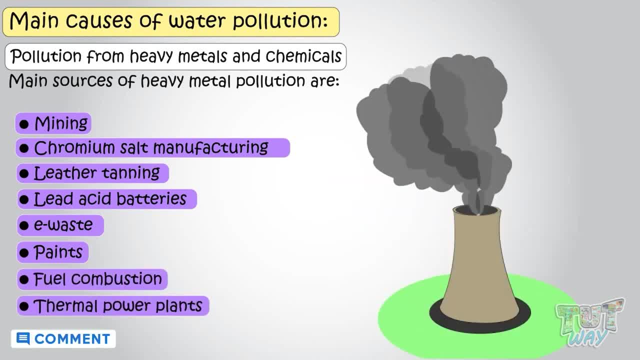 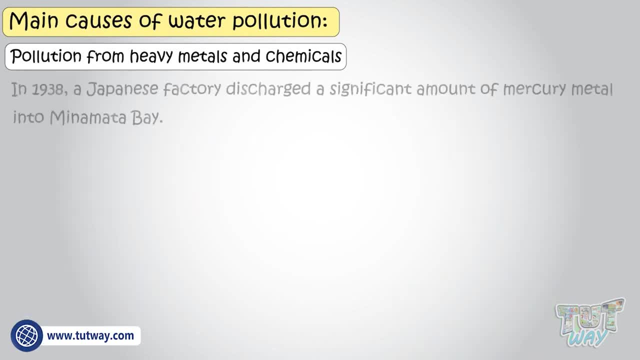 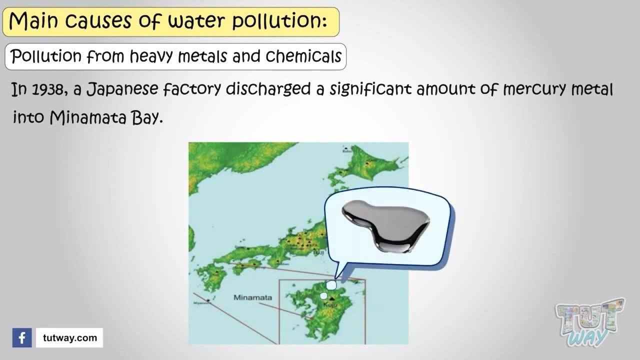 Combustion And thermal power plants. The best known example of heavy metal pollution in the oceans Took place in 1938. When a Japanese factory discharged a significant amount Of mercury metal into Minamata Bay And that led to the death of so many fish. 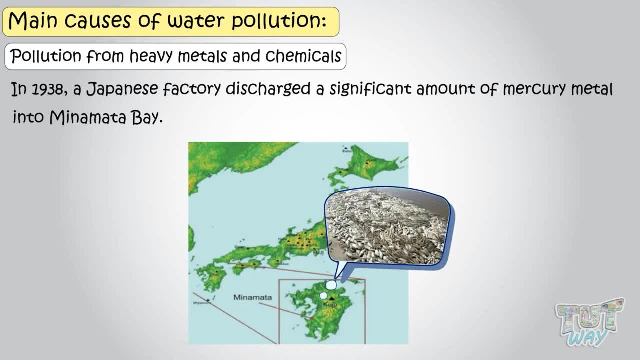 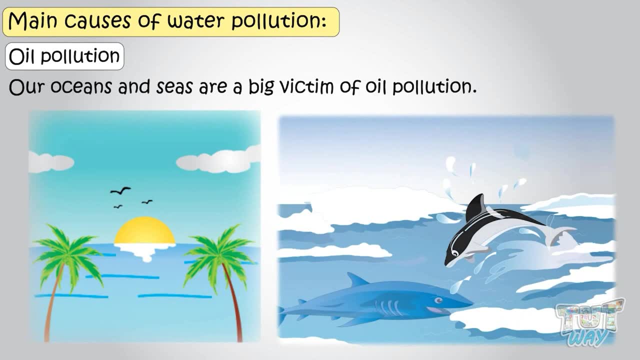 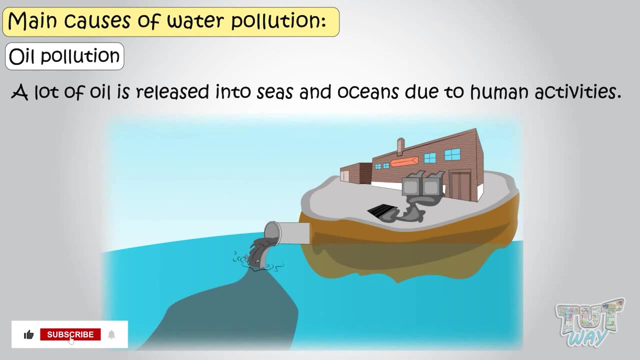 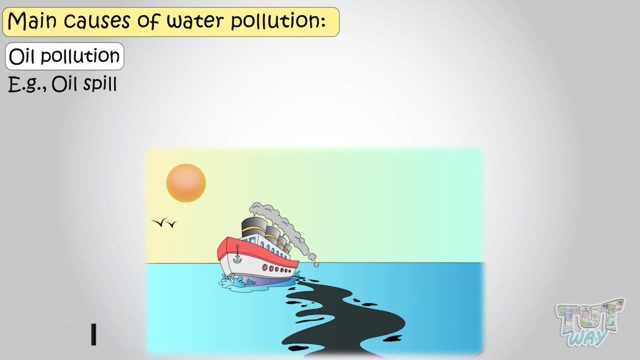 Next is oil pollution. Our ocean and seas are a big victim of oil pollution, As a lot of oil is released into seas And oceans due to human activities, Like oil spills from huge oil tanks And ships. Oil spills is a major problem. 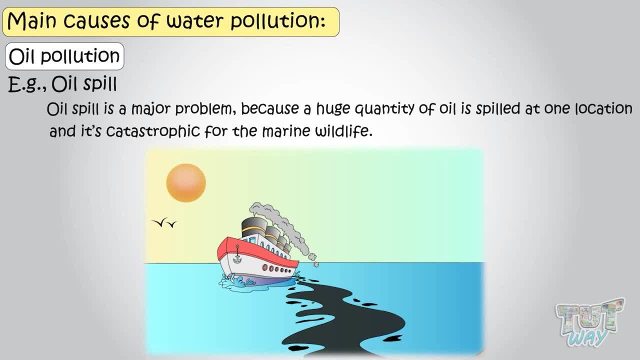 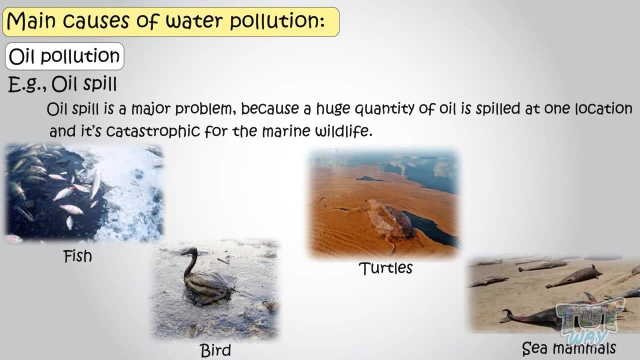 Because a huge quantity of oil Is spilled at one location And is catastrophic for the marine life, That is, many species of fish, Birds, Turtles And sea mammals. Oil pollution is not only a result of oil spills, But a lot of oil in sea waters. 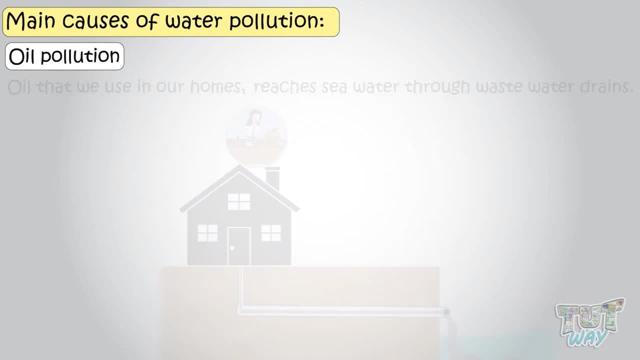 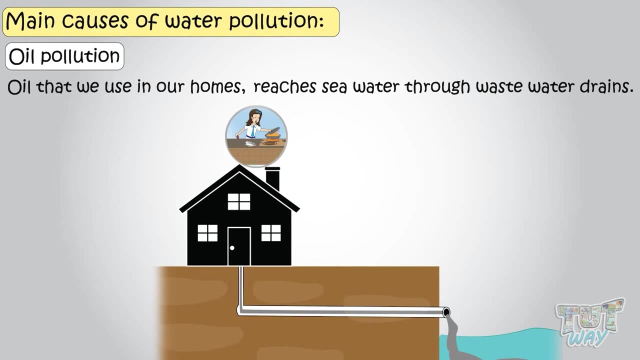 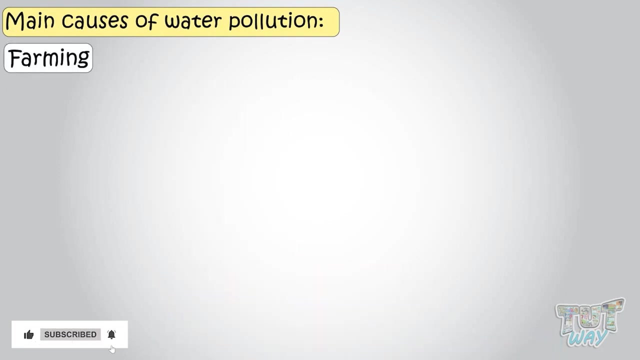 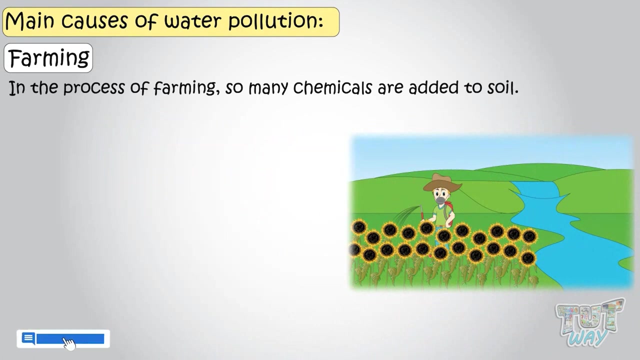 Comes from routine shipping. Oil that we use in our homes Reaches sea water through waste Water drains. Another source of water pollution is farming- Yes, farming. In the process of farming, too, So many chemicals are used, Like pesticides are used to kill pests. 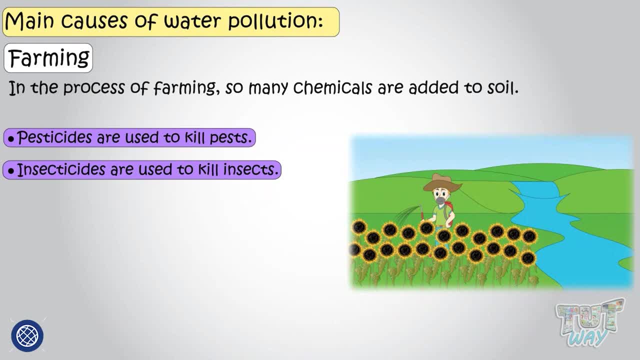 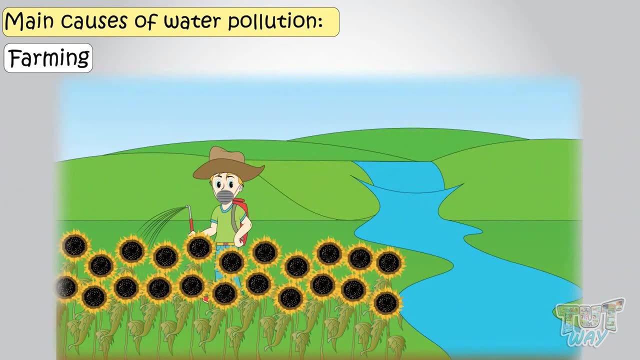 Insecticides for killing insects, We decides, are there to kill the unwanted plants. Fertilizers are there To make the soil more fertile. All these things contain chemicals That ultimately reaches the ground water And pollute it, And also.